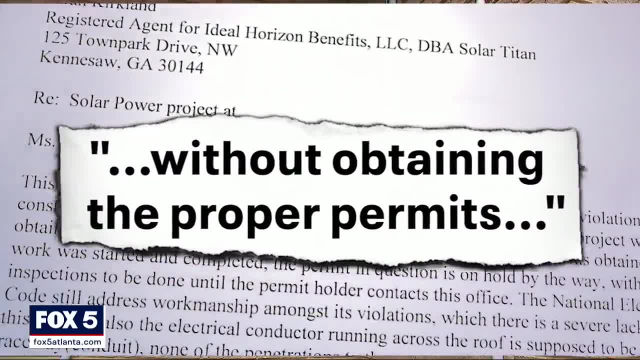 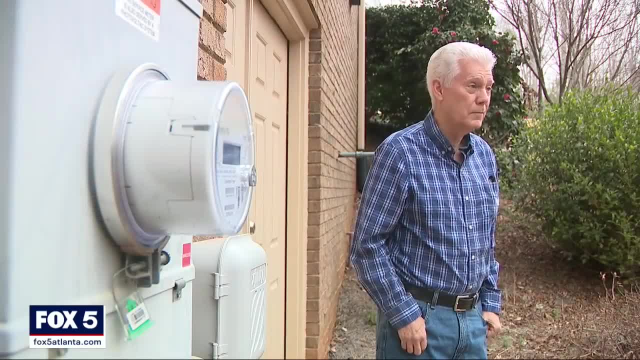 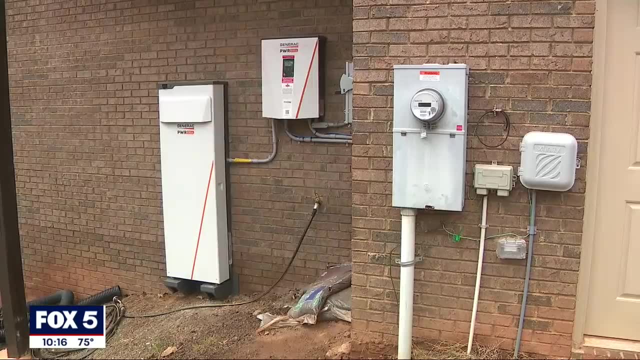 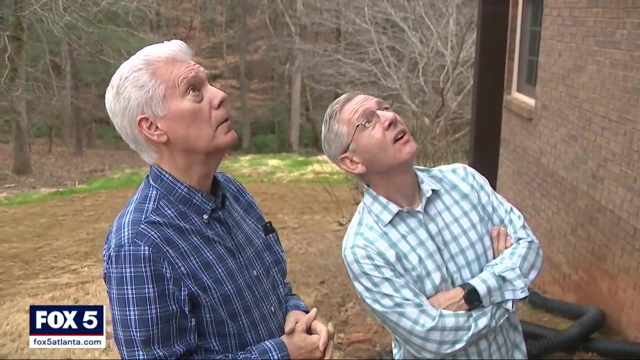 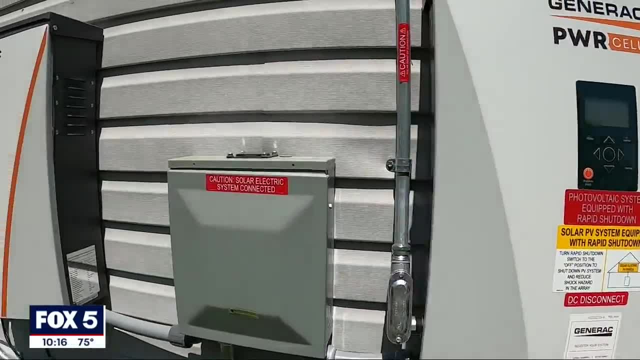 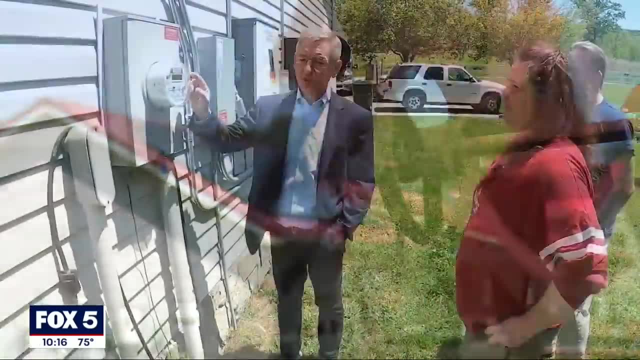 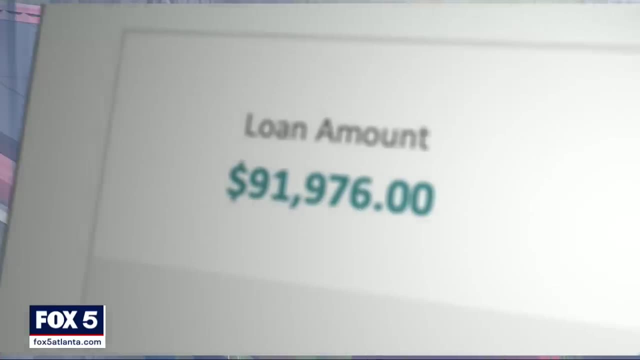 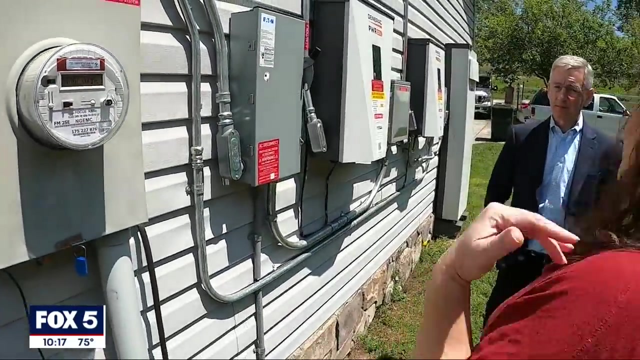 Everything he said turned out to not be true, Like how Amy and Nathan Tetra would be able to sell extra solar power back to their utility, thus giving the Lafayette couple a negative electric bill. Have you seen a negative power bill? No, never. Their power home solar system cost $91,000, financed over 25 years. Her North Georgia EMC bills have barely budged. If I'd have known all this, I would have never made this decision. I would have just stayed with my regular old power company. 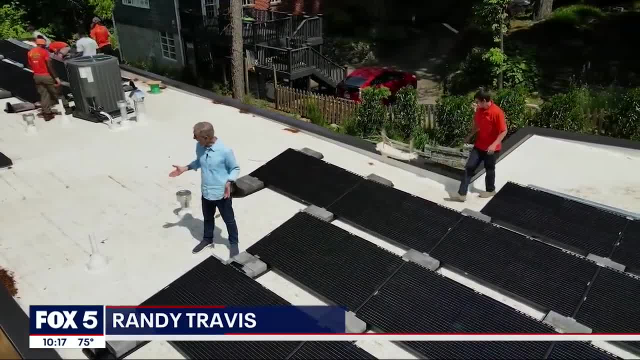 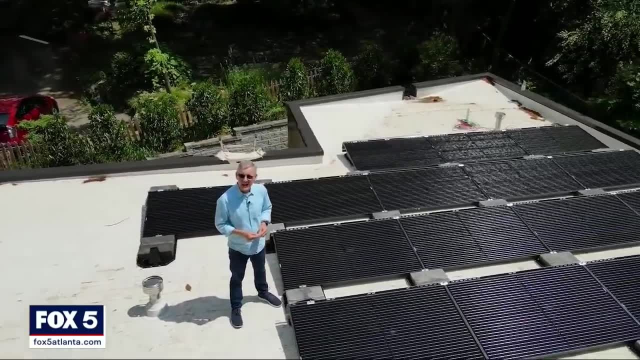 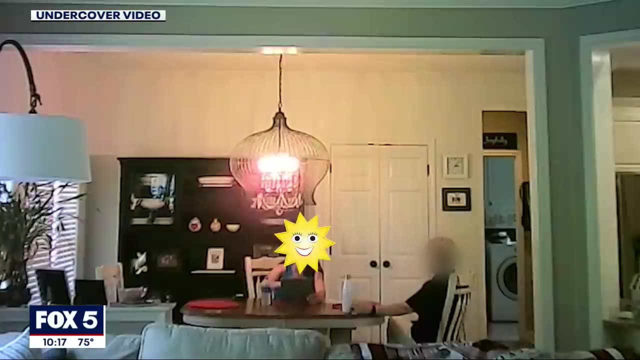 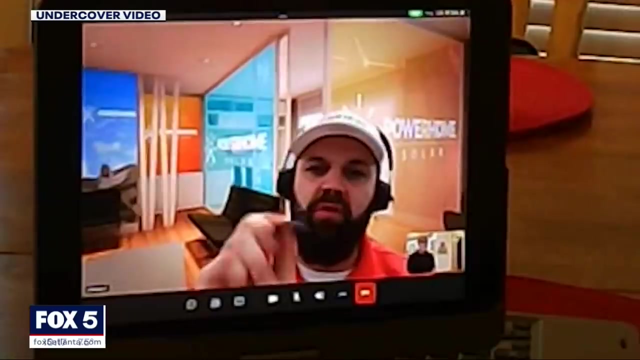 It's an understandable feeling. For some homeowners, solar power is a legitimate option if they want to try to cut back on rising energy costs. But many of them don't know the right questions to ask. Well, we do know the right questions, But listen to the answers we got. Power home solar decided not to use their happy salesperson to make the hard sell for us. Instead, we were patched in to speak virtually to Andrew, who said he was a senior account manager. So we're showing his face. These are expensive. 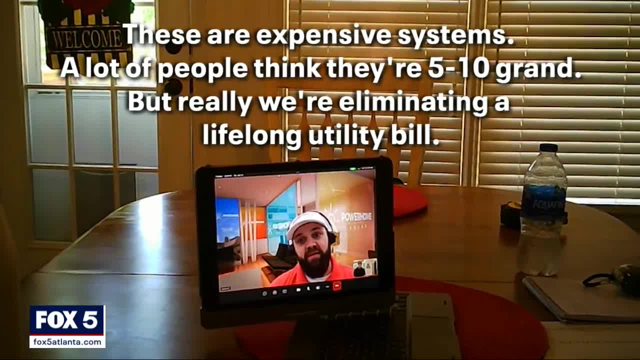 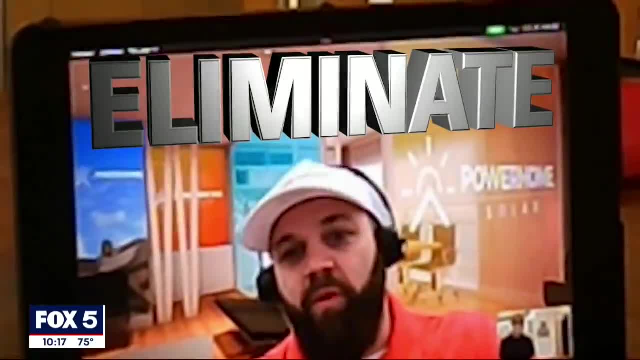 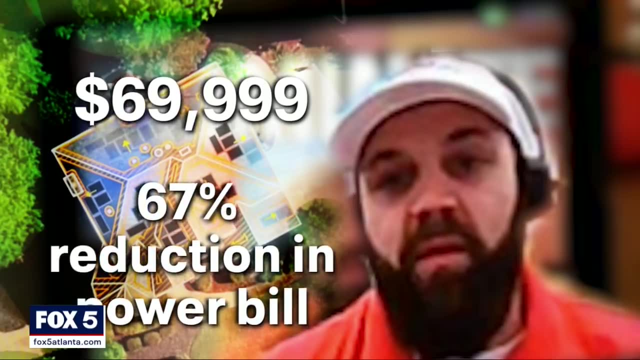 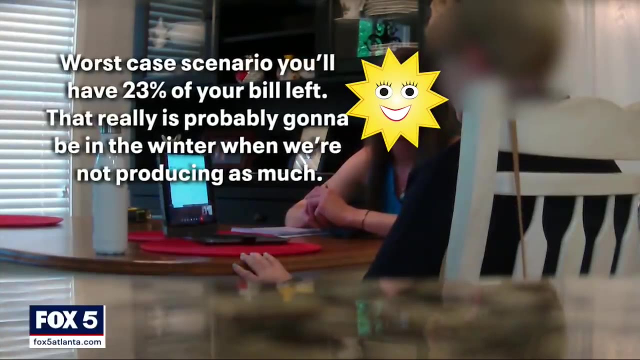 systems. A lot of people think they're five, 10 grand, But really we're eliminating a lifelong utility bill. That's right. He said: eliminate. To do that, Andrew quoted us $69,999, later guaranteeing a 67% reduction in our power bill. Worst case scenario is you'll have 23% of your bill left, But that really is probably going to be in the winter when we're not producing as much. 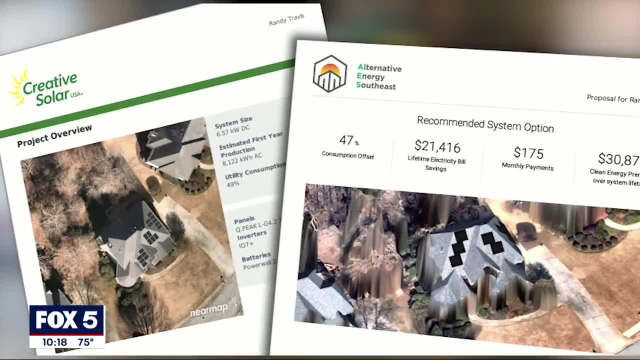 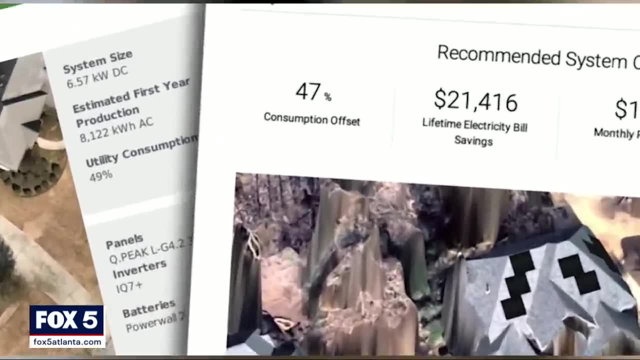 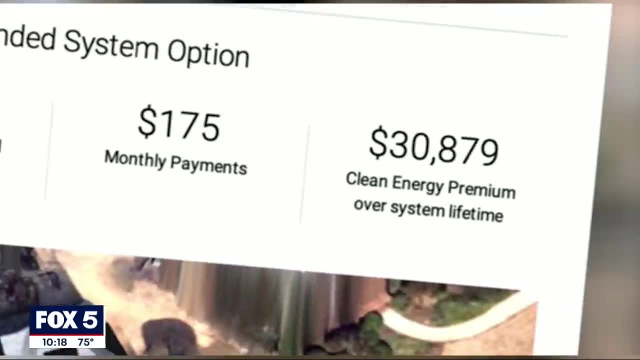 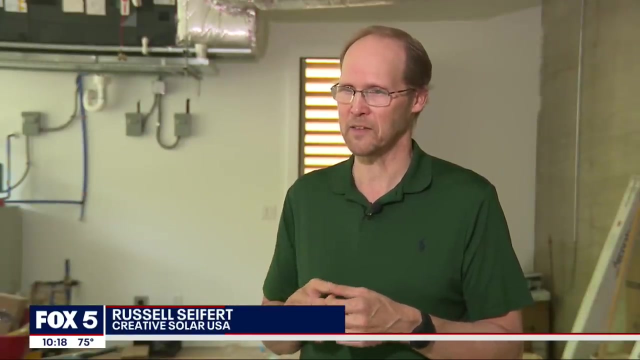 We had two local companies design solar systems for the same house: Creative Solar USA and Alternative Energy Southeast. Because of shade and the roof design, neither said it would reduce our utility bill by 67%, not even by 50%, But their cost was drastically lower than power home solar's price And this is why it's good to get a number of quotes to compare. And then the truth serum comes out. You also have one to one net meter, which is huge. 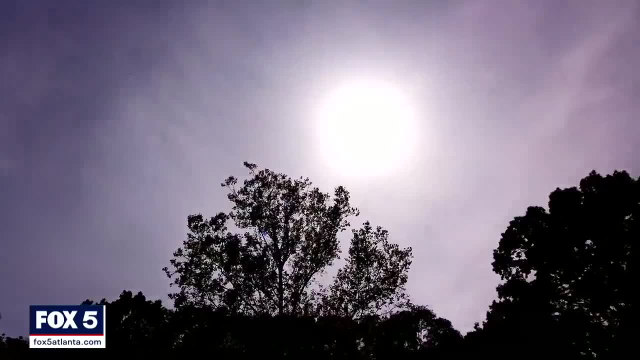 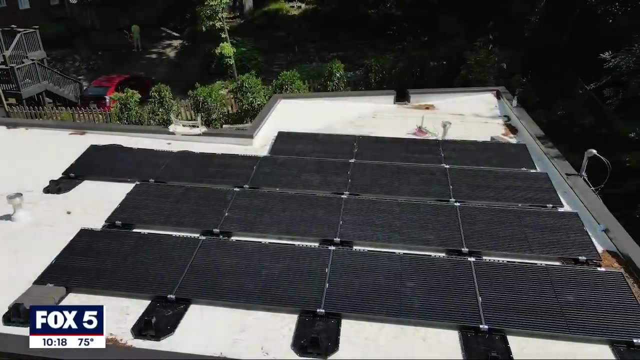 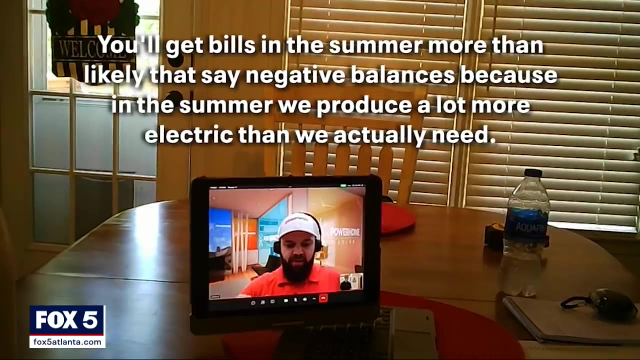 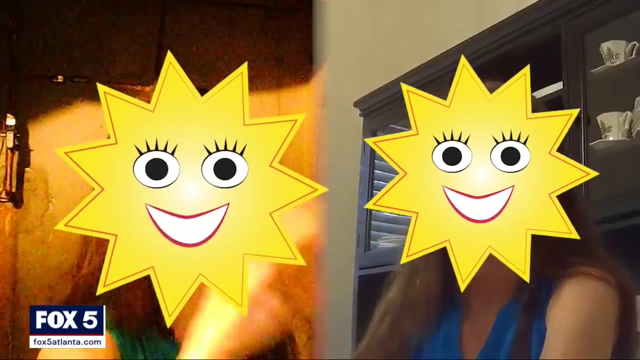 Andrew Ronley promised that we get full credit for every unused solar kilowatt we sent to our electric company. It's called net metering and can reduce your electric bill dramatically. You'll get bills in the summer more likely that say negative balances, because in the summer we produce a lot more electric than we actually need. But Walton EMC, the utility that services this home, doesn't offer net metering. Power home solar said it fired Andrew because what he told us didn't work. 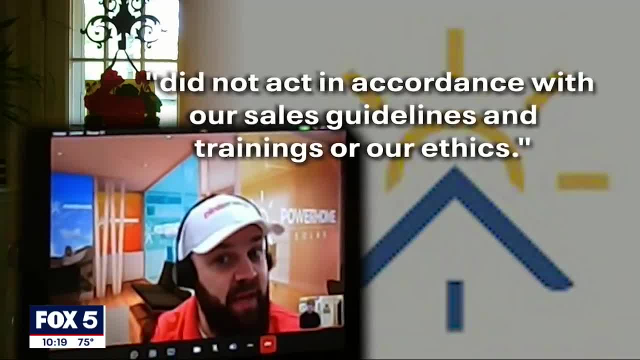 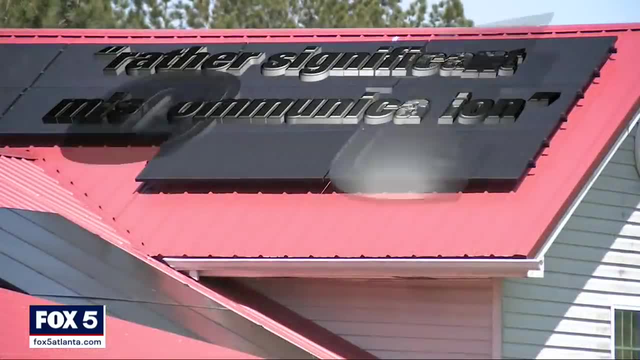 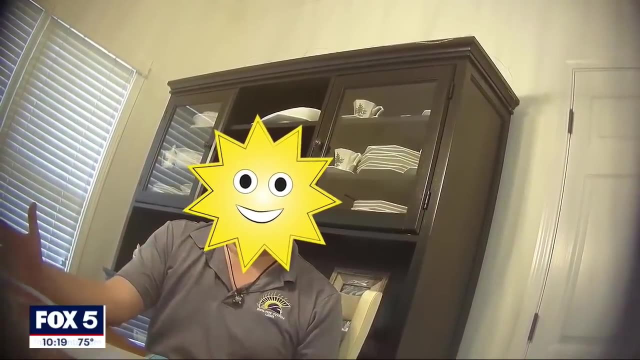 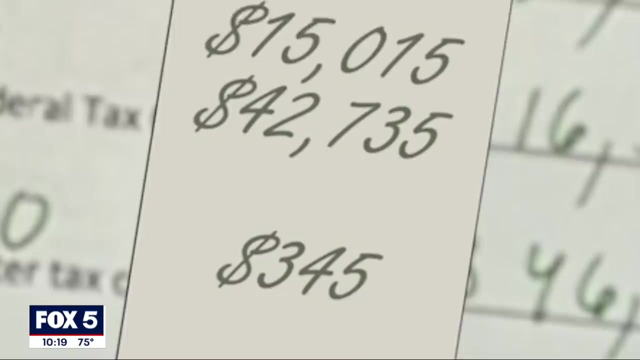 They also agreed to cancel Amy and Nathan's contract and take down their system against, citing a rather significant miscommunication by their sales rep. It's almost going to be harder and harder to get solar in the next couple of years. Solar Titans recommended estimate for our house was almost as high, nearly $58,000. That's $345 a month for 20 years. Am I still going to pay for power? No, 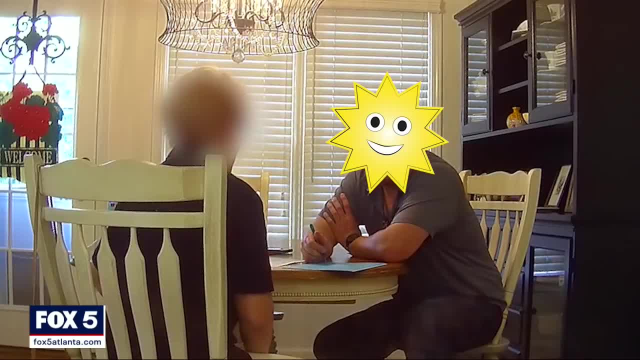 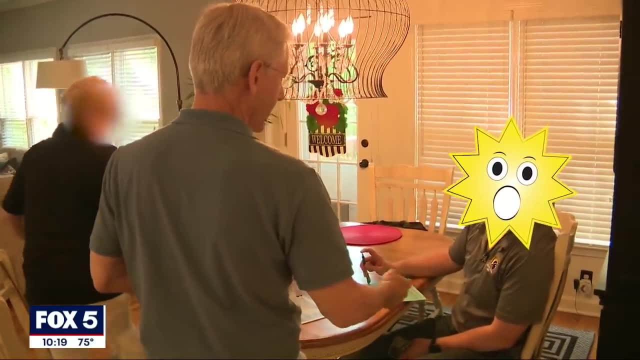 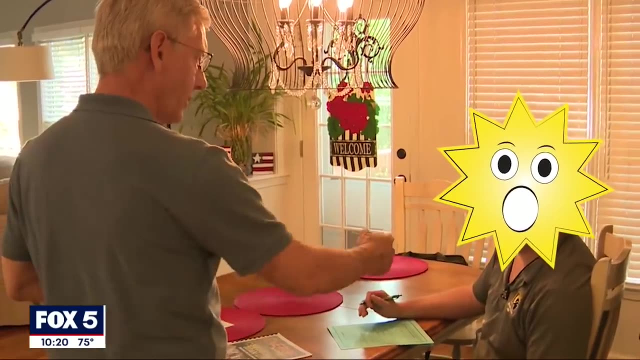 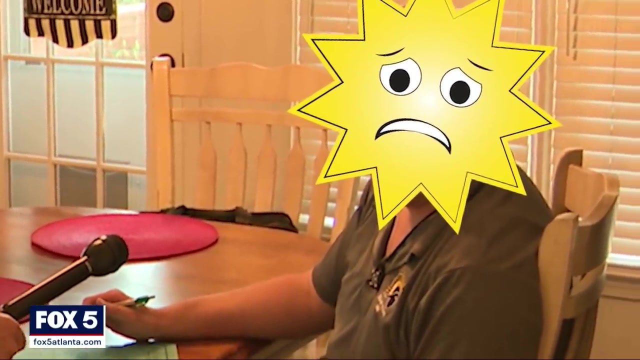 No, that's the So with this. this is right here. You'd pay this to take care of all your all of your usage. So this would be about 100% of your usage right now. Randy Travis, with Fox 5 News We've had some complaints about your company, So we want to kind of hear how the sales pitch went. How can you promise her that her power bill have no consumption charge at all with this unit? How can you make that promise? I'm not going to answer any questions from you, man. This is real uncomfortable for me. Well, imagine the people who have been told that and they get power bills even after they spent some money on it.